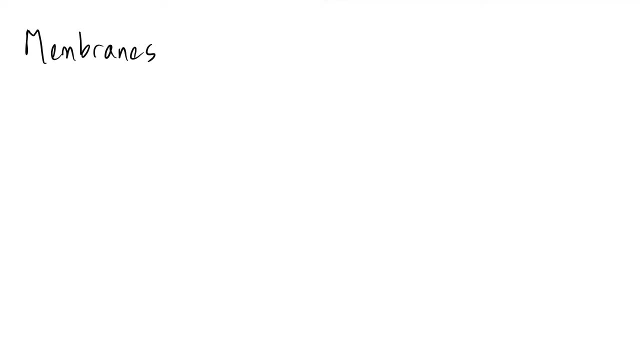 kind of utility from it, And a generic example or how membranes are represented on process flow diagrams is something like this. So we'll have some kind of unit, we'll have a membrane within this unit, we'll have a feed entering, we will have a retentate stream that makes it over the 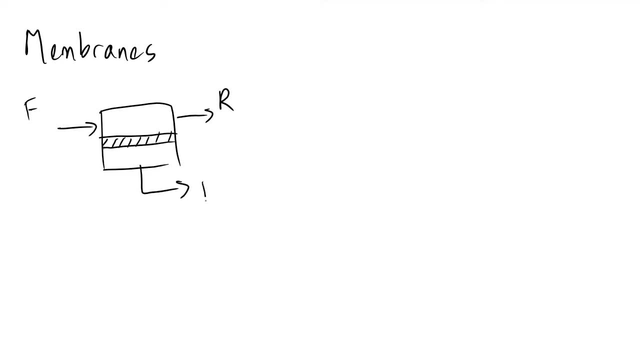 membrane and then we'll have something referred to as a permeate stream p, And the permeate stream is what actually it's passed through the membrane. And to give an example, if we had some kind of size exclusion- membrane particles smaller than the pore size- 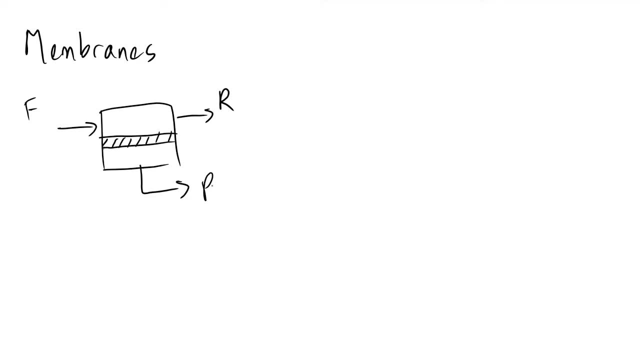 of our membrane would be concentrated in our permeate, And at this point it is a good question to ask: what kind of flux can we be expecting from our membrane? As in, what kind of flow- molar flow- can we expect from our membrane? And at this point it is a good question to ask. 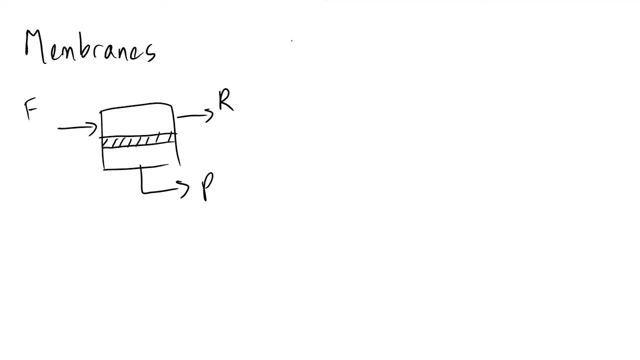 what kind of flux can we be expecting from our membrane, As in, what kind of flow, molar flow rates can we expect in a given unit? And so, writing this out, what is flux? So this will depend on the kind of fluid that we're using. So for a gas, we'll be working with partial pressures. 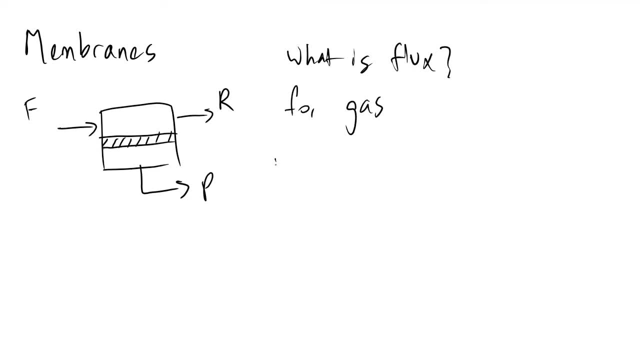 and Henry's coefficients And the flux of some component i across our membrane. so the quantity per area per time the membrane will have some known area will be equivalent to h sub i- sorry about the handwriting. the Henry coefficient for that particular component i times d sub i, the diffusivity of that component. 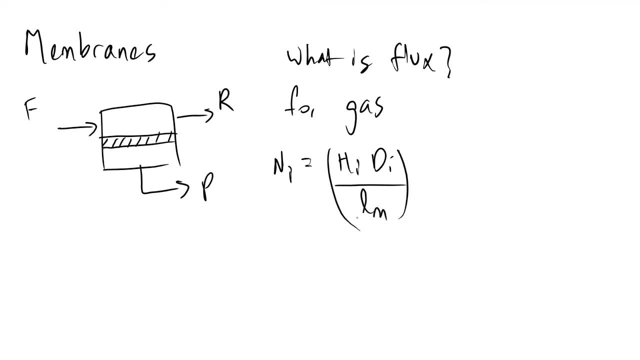 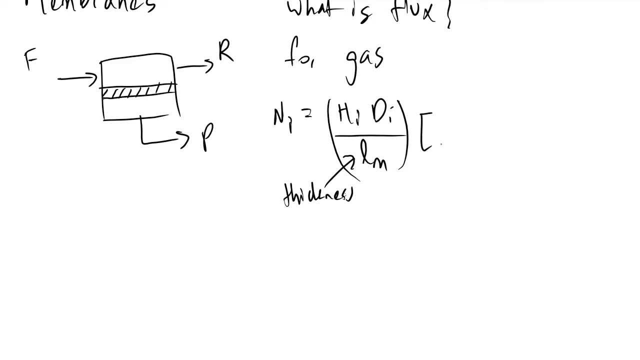 divided by L sub m, which is the membrane thickness times the driving force, which will be sorry- will be equivalent to the difference in partial pressure between the two sides of the membrane, So partial pressure of component i on the retentate. 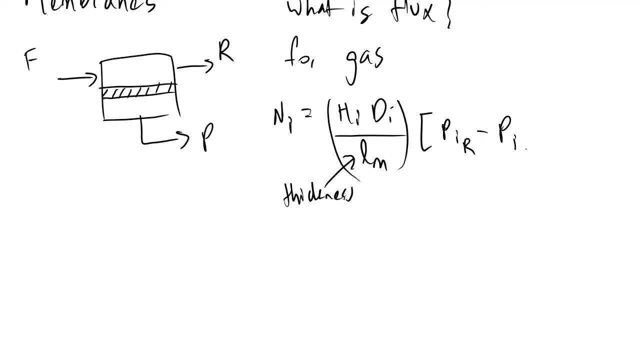 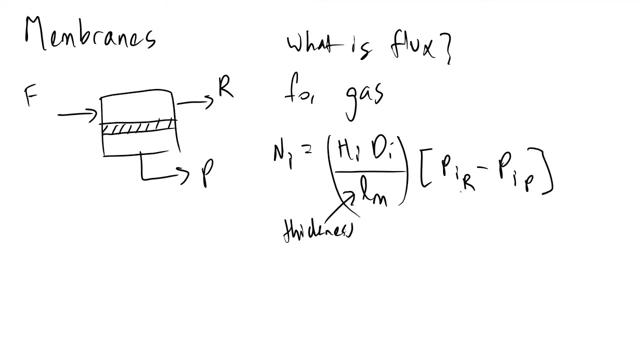 side, minus partial pressure of i on the permeate side. And if we are working with systems in which the it is not well mixed on the retentate side, then we will see that it is not well mixed on the feed or retentate side. this sorry p sub i r term can take on will be some kind of function. 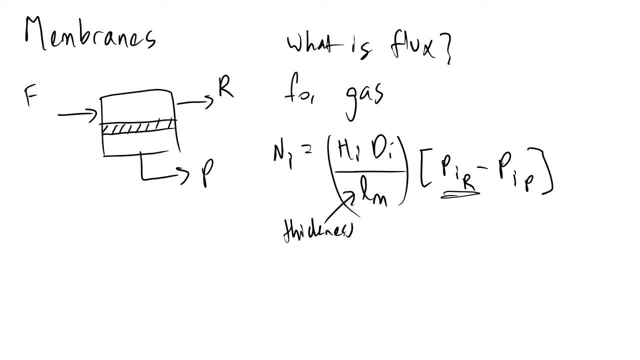 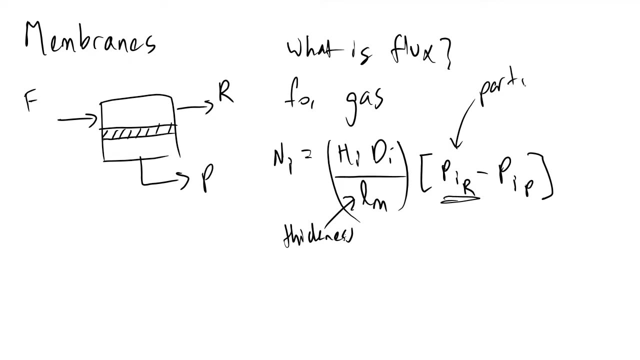 of the accumulated length of our membrane, And so what we can do is just take an average value of that, if we know that quantity, And just to write this out, this term here will be the partial pressure of component i on the retentate side. Okay, and so this is the molar flux equation that 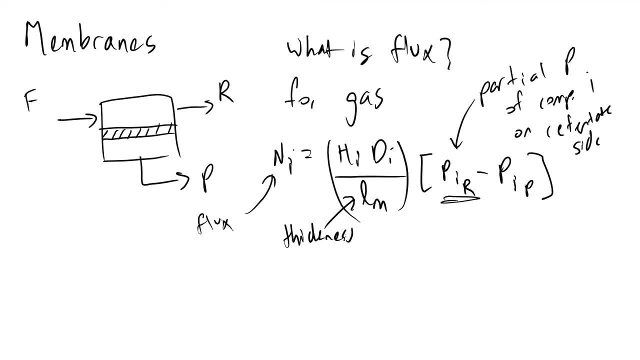 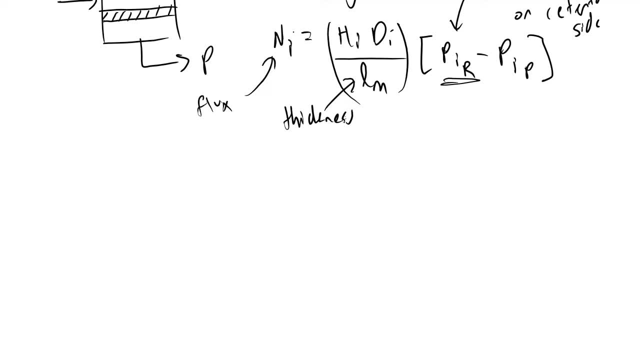 we will use for gases. Now for liquids, things will look mostly the same, except instead of partial pressures and Henry coefficients, we will be using equilibrium constants and concentrations, And so the flux- sorry flux- for liquids will be equivalent to n. sub i is equal to. 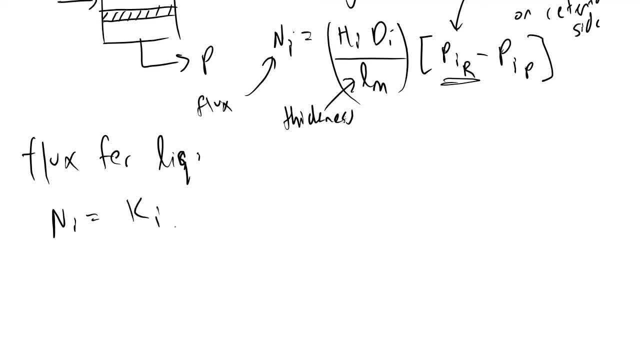 n sub i, K sub i, the equilibrium coefficient for component i times the diffusivity of component i divided by the membrane thickness times the driving force, which is the difference in concentration of component i between the retentate and the permeate side. And at this point I would like to note: 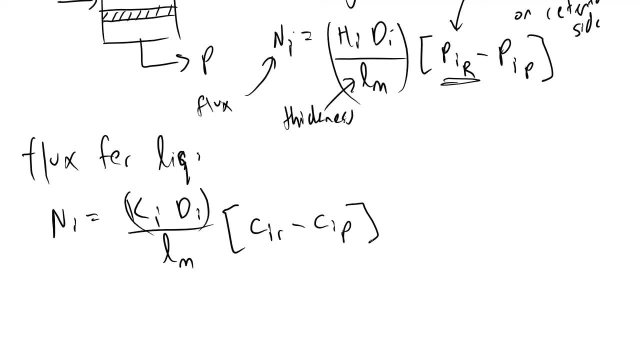 the definitions that you'll commonly see, such as permeance and permeability, And you'll note how, in these two flux equations for liquid and gas, we have the quantities h sub i, d, sub i and k sub i, d, sub i. 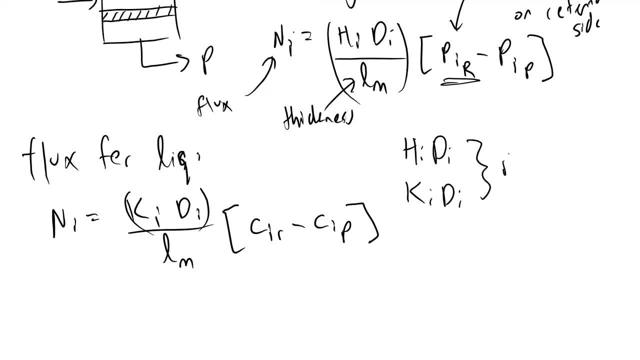 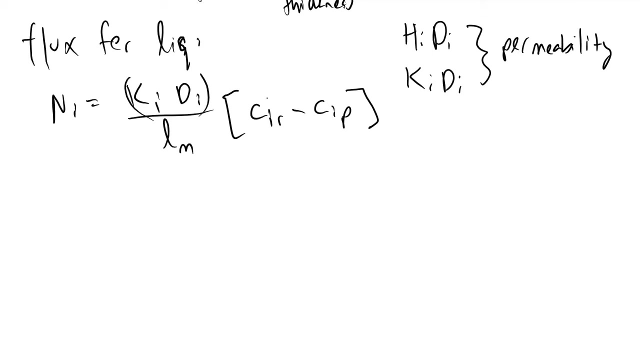 These terms by themselves are permeabilities, And permeabilities will take on unique units you can find in textbooks And like any other flux equation, we know that flux is equal to some coefficient times the driving force. The permeability is not that coefficient, but the permeance is. 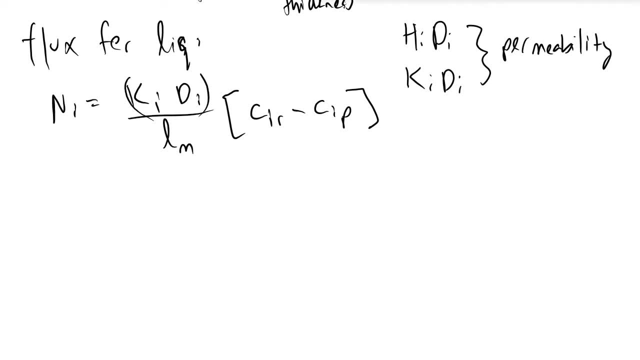 And so if we and so our permeance will essentially be equivalent to the permeability of the liquid, This term, the term in front of our driving force in our two flux equations for liquid and gas, And just to clarify, our permeance is generally equivalent to, like some kind of mass transfer coefficient. 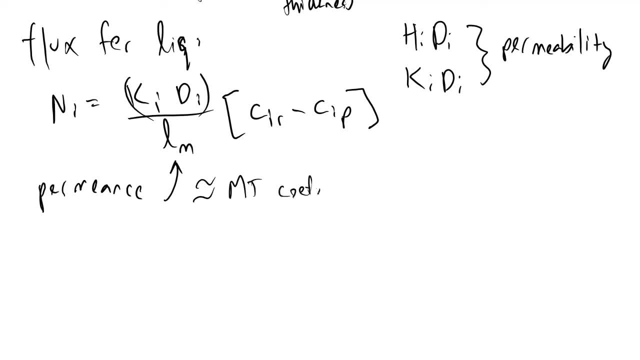 like we've seen previously in our flux equations And moving on, we I will go into some typical equations that we will come across. We'll go into some typical equations that we will come across When trying to solve membrane problems. Usually what we will be given will be the feed molar flow rate. n sub f. 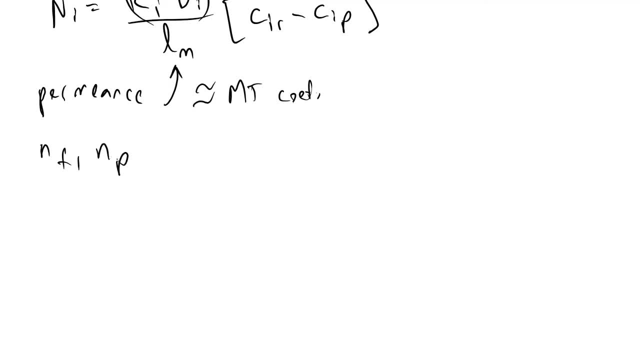 The permeate molar flow rate n sub p, Something called theta, which is the cut, As well as the composition of our feed stream, of some component that we are interested in, And the thing to note about theta is that theta is equivalent to the flow. 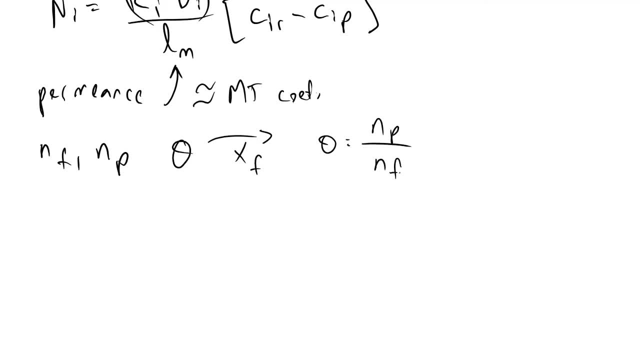 the molar flow rate of our permeate stream divided by the molar flow rate of our feed stream, And so our cut can take on any value ranging from zero to one. When theta is equal to zero, it means we have no permeate stream. 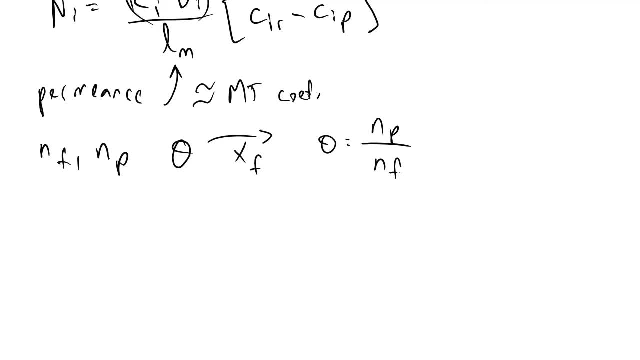 Our membrane is somehow completely impermeable. Nothing's getting through it, And so our feed stream is the only thing that's going to get through it. Our feed stream is the only, or our retentate stream will have the same molar flow rate as our feed stream. 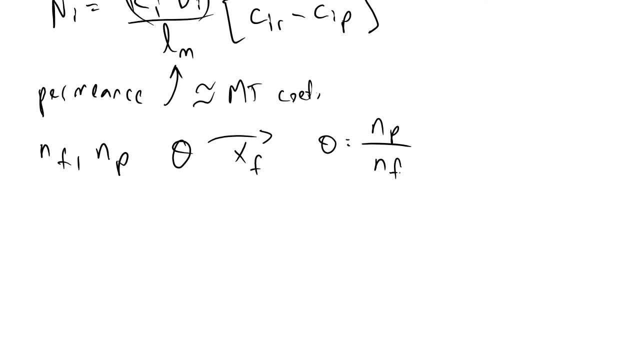 Assuming there's no reaction occurring, And applying mass balances on our membrane results in equations such as this. So if we were to do some kind of component mole balance on some species A, for example, What we would find is that the retentate composition of species A is equivalent to the feed composition of that species A minus. 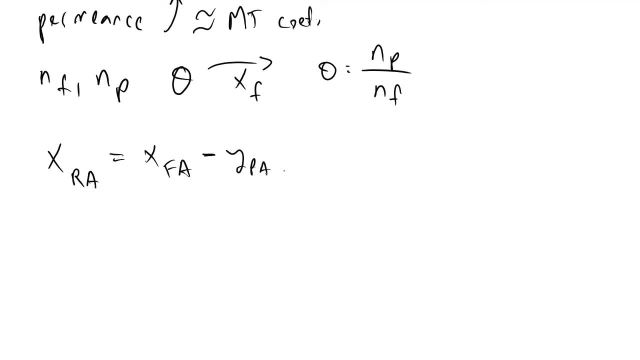 the permeate composition of that species A times the arc cut, and this quantity is divided by 1 minus theta. So this is a common equation you'll use from the mass balance, and these mass balances can be a little bit tedious to do, so typically we'll just go right. 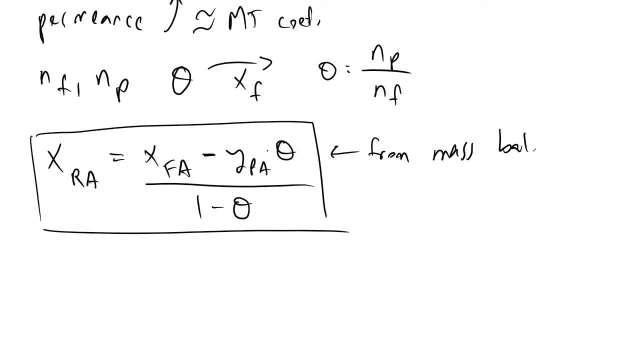 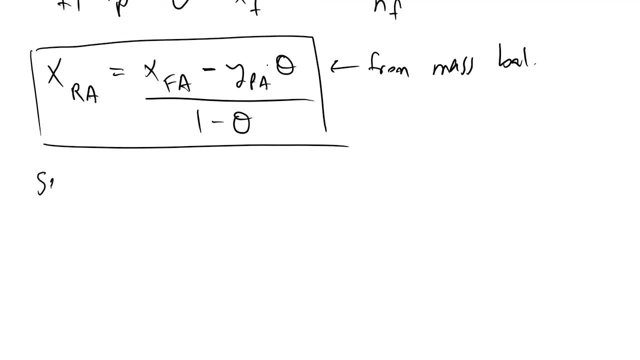 to the equation and use it to arrive at some final result. We also define a quantity, referred to as a separation factor, that is commonly used in membranes, and the separation factor is called alpha AB, and so, assuming we were working with some kind of B-type membrane, we're going to use alpha AB as the separation factor. 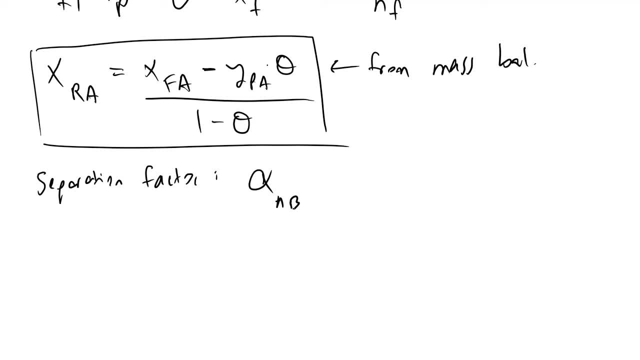 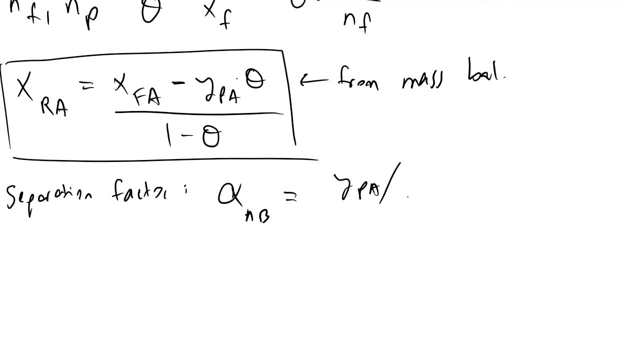 binary system. it tells us the separation factor for this particular system and it is equivalent to the permeate composition of species A divided by the retentate composition of species A divided by 1 minus the permeate composition of your species A. and that quantity is divided by 1 minus XRA, so the retentate composition of your species A. 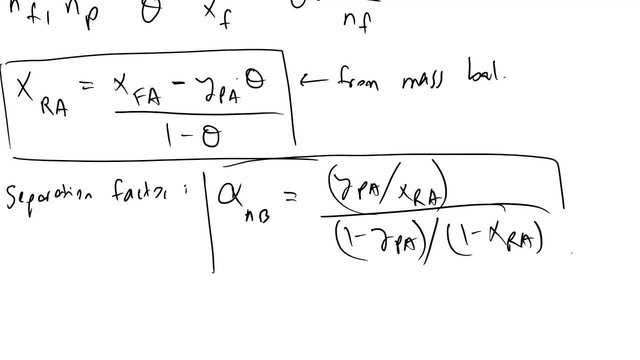 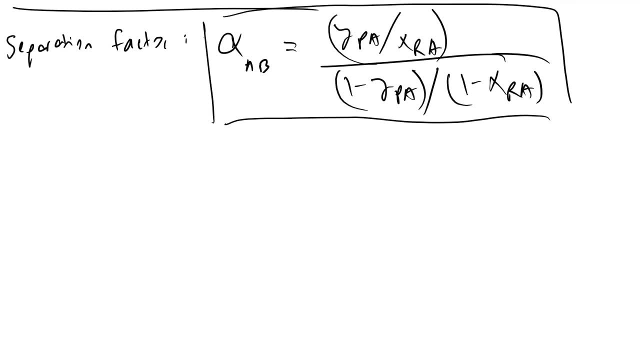 And a final equation that will typically come in handy when we are working with membranes is the definition of another variable referred to as selectivity, and selectivity is an intrinsic property of the membrane itself. So when you go to a membrane manufacturer and you have some kind of requirements, it will be unique to the membrane and it will make a membrane quite. 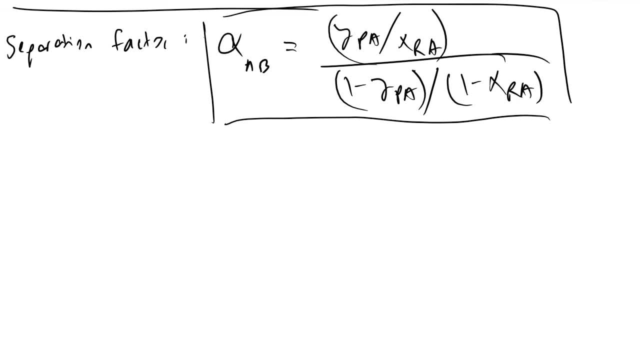 expensive, And the selectivity value is a function of the separation factor that we just defined. It is the way we evaluate our selectivity, which is alpha, AB, star, which is this quantity here is through this equation: In the case of a cell membrane, the selected structure is the other cell in the cell. So we can do that. We also have to find how to measure the selection of membrane selectivity. So we have these two equations, alpha, AB, star, and this quantity here and this equation, And this equation is called selection of membrane selectivity. 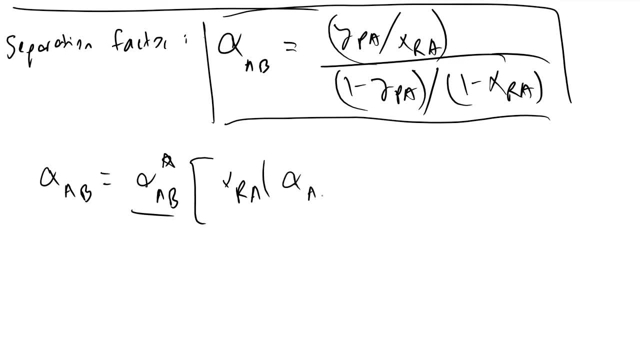 And I'm sorry for just writing out these equations, but the math is from derivations that you can find quite readily in textbooks, And usually in these kinds of chemical engineering classes it's mostly the application of these equations. So we're gonna divide this quantity by and sorry. 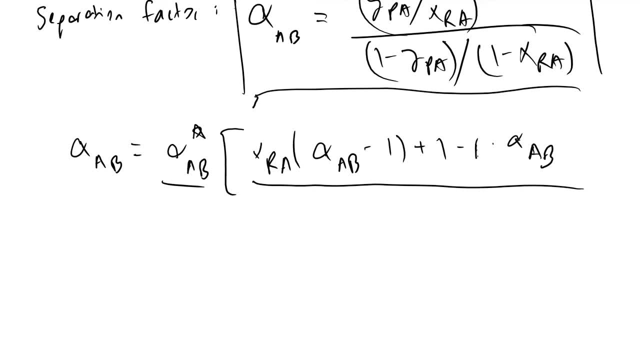 I will define. so this variable right here is r, and what I will do is finish writing this up. Okay, and so this quantity here is equivalent to our selectivity. You may likely be asked to find it on an exam if you are given the separation factor. 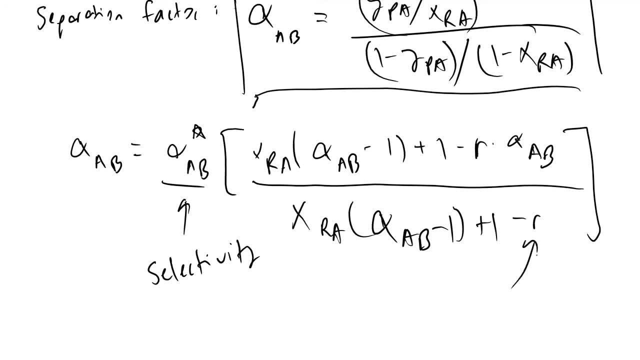 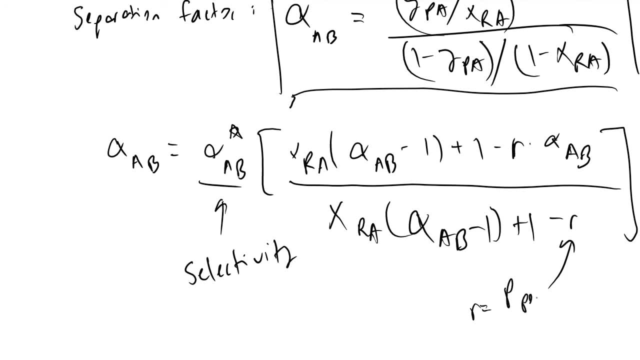 and this term r is a ratio of the pressure in our permeate divided by the pressure in our retentate or, I'm sorry, in our feed or retentate side. And so if we assume that our feed and our retentate, 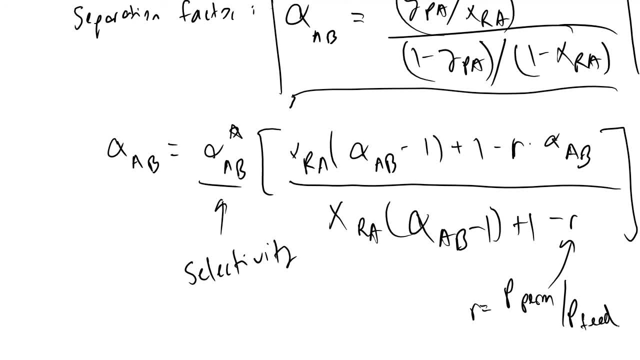 have the same pressure, that would be equivalent. So generally the maximum pressure ratio we can have in practice is typically about five to one. So our permeate would be 1, 5th or five times greater or less than the pressure on the opposite side.